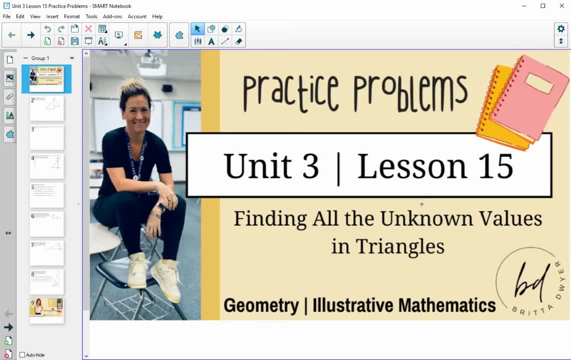 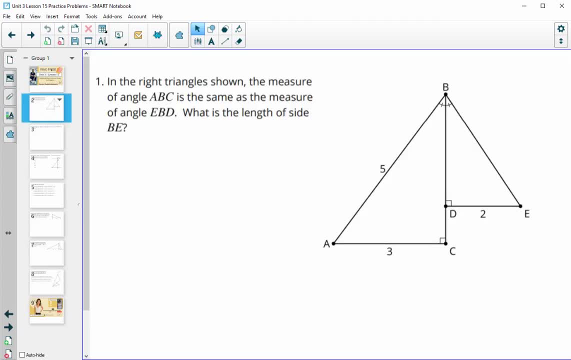 In this video we will look at the unit 3, lesson 15, practice problems. Number one tells us that we've got two right triangles shown and then that the measure of angle ABC- this one right here- is the same as the measure of EBD. this 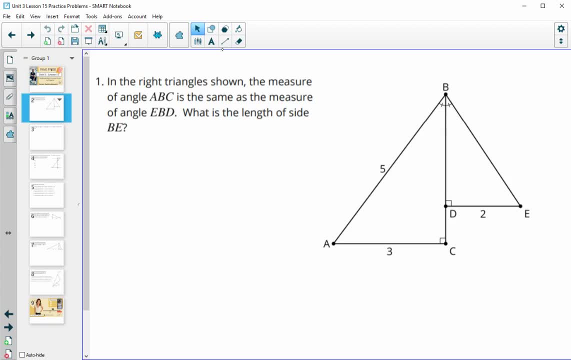 one here, and we can see that they marked that as well, and now they are wanting to know the length of segment. be, so we're looking for the length of this segment. this segment corresponds to this one, and we know that these triangles are similar because they have two angles the same, so we'll be able to set up some proportions. 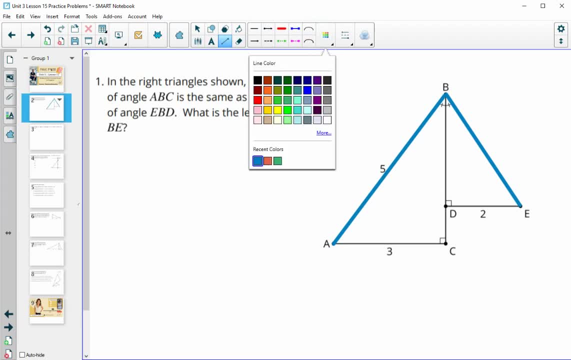 here or use scale factor. so if I take a look, I also see this side and this side are corresponding and they're are filled in with numbers. So this will help me to get the scale factor. So I'm going to be wanting to take this number and multiplying it by something. So we're going to look at the scale. 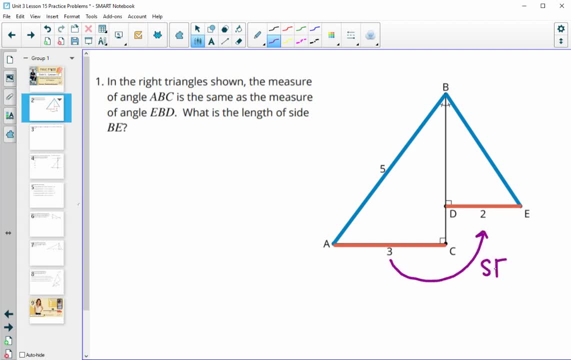 factor that takes three to two. So that scale factor will be two divided by three. So our scale factor is two thirds. So in order to find B E, we will just do five times the scale factor of two thirds And then that will give us that side B C is 10 thirds. So you could write it like that. 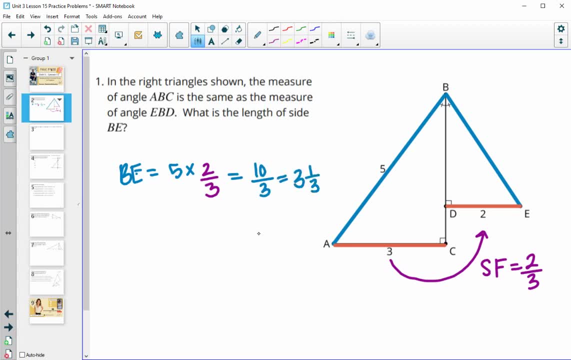 You could write it as a mixed number of three and one third, or you could write it as a decimal of 3.3 repeating. So any of those are fine. You can also set up a proportion, if you would like, versus using scale factor. 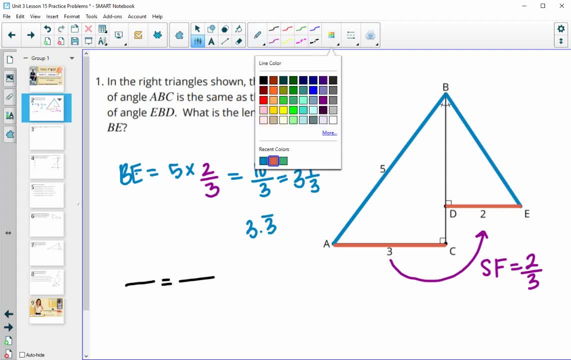 So if you were doing proportions, you might start with this side, So putting X with its corresponding side of five, and then choosing from this same triangle, here you could put two and then its corresponding side three, And then, if you cross, multiplied, you'd again get 10. 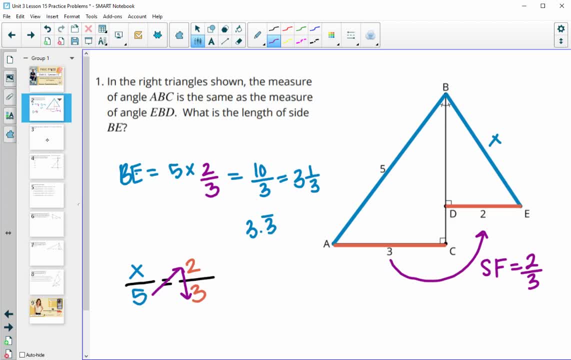 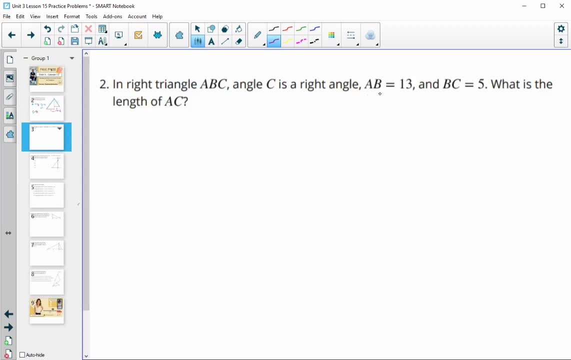 divided by three, It's going to come up with the same answer either way. Number two in a right triangle, ABC, angle C is the right angle, And then it gives us two of the side lengths and wants to know the third. So if we go ahead and just draw ourself a right triangle, 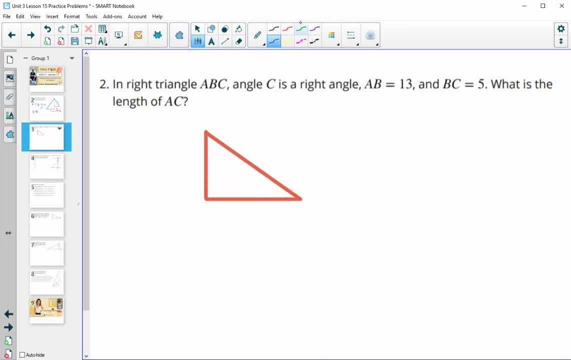 so that we can label it. it told us that the right angle is letter C, So then you can put A and B wherever you want on these other two And then if we go ahead and just draw ourself a right triangle, so if we go ahead and just draw ourself a right triangle, and then we get that we're right on this left triangle. 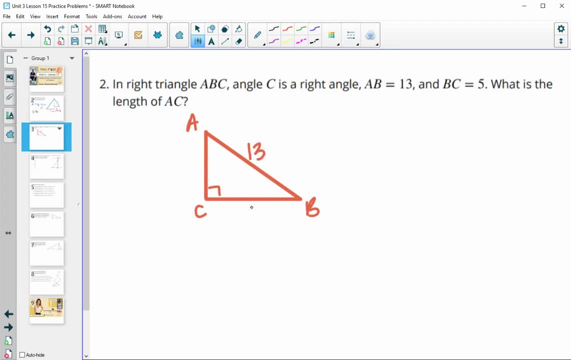 So A- B, the hypotenuse is 13.. B, C is five and we're looking for A C. So we'll do the Pythagorean Theorem. So we know that Pythagorean Theorem is the hypotenuse squared is equal to the two legs. 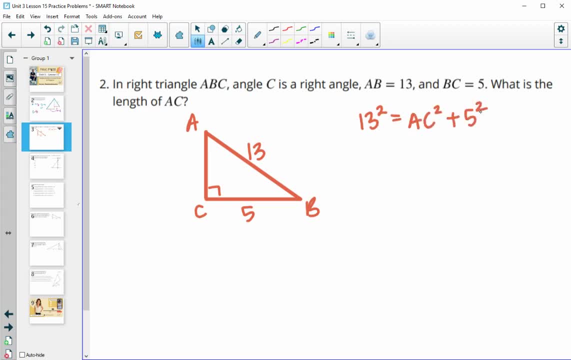 A, C and B, C or five squared and added together, So we'll square the hypotenuse 169.. We still have this missing side squared and then plus five squared, which is 25 subtract 25 from both sides, and you get that AC squared. 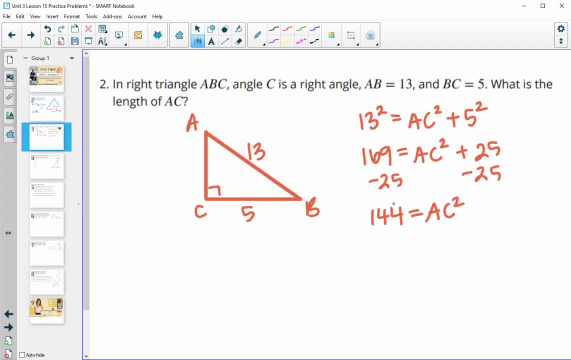 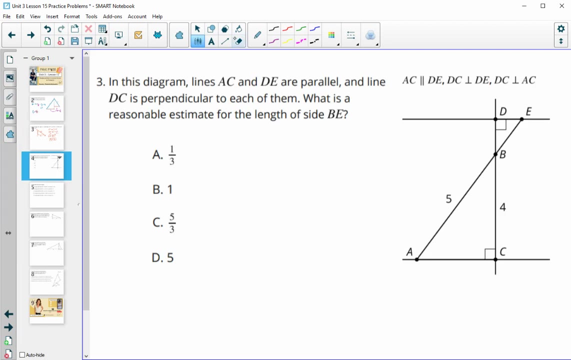 is equal to 144. so then we will square root and you end up with: AC is equal to 12. number three tells us that we have a diagram with some parallel lines. so we know that de is parallel to A, C, and then we know that DC, going through here, 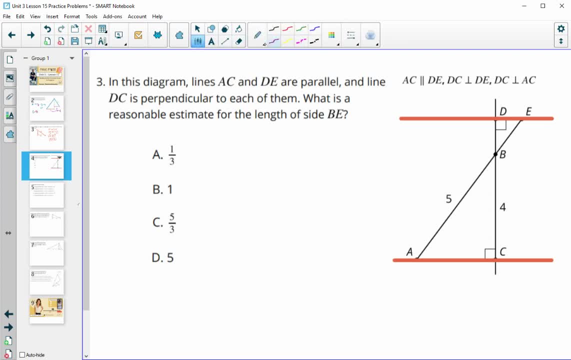 gives is perpendicular to each of them. so then they want us to know what would be a reasonable estimate for side be, and so be is here, and so we're just estimating, because we don't know the coordinate and the degree of the know any of the lengths in this little triangle, so we can't set up proportions. 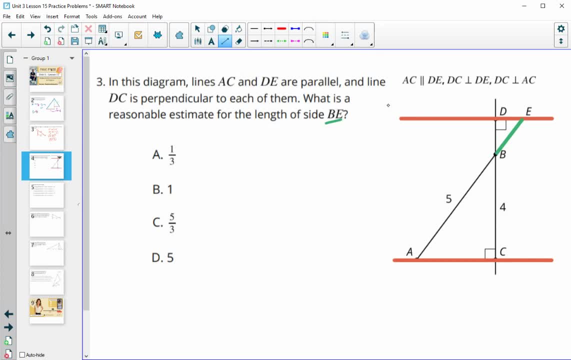 but we're just trying to come up with a reasonable guess. so we know it's gotten smaller, since these triangles are similar. okay, because we've got a vertical angle here and the right angle, so we and we can see it's gotten smaller here. so five wouldn't make sense and it doesn't look like it's less than one. 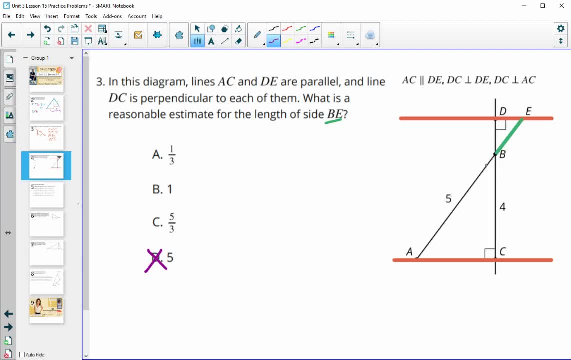 unit. okay, because this is five and this would fit in there at least a couple of times. not, it's not going to fit in there more than five times. this segment doesn't look like it'll fit in there five times, so it doesn't look like it's. 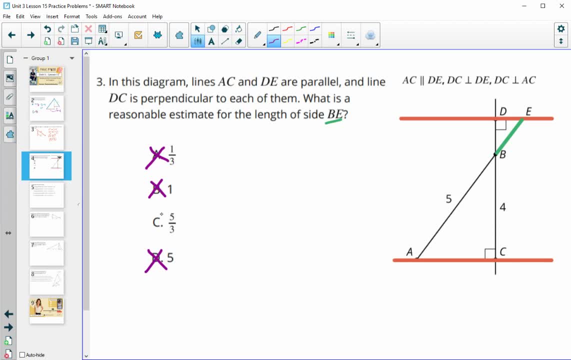 less than a unit, or even just one unit. um, so I think five thirds is probably the best estimate. so looks like it's about one third of the size. okay. so if we look at this, here's one, two, three. it looks like it's less than a unit and it's not going to fit in there more than. 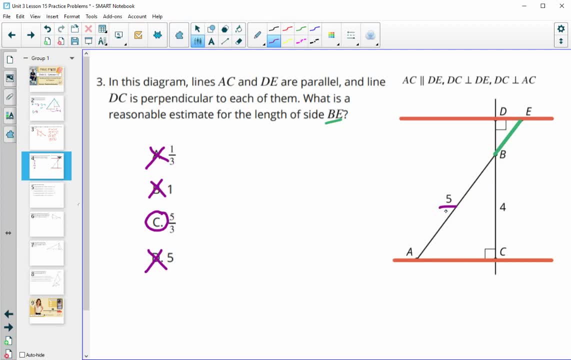 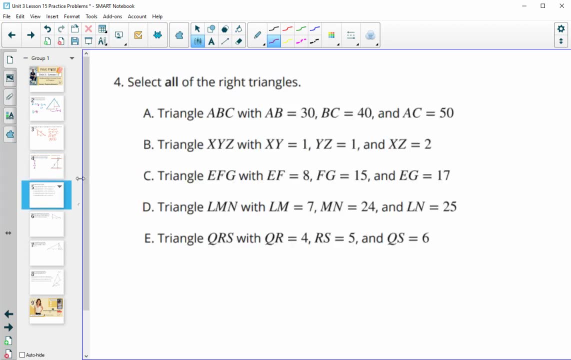 like that segment fits in there about three times. So if we took five and divided it into three equal pieces, looks like that would be a good guess. Number four: which of these triangles are right triangles? So remember that we will do Pythagorean theorem that a squared plus b. 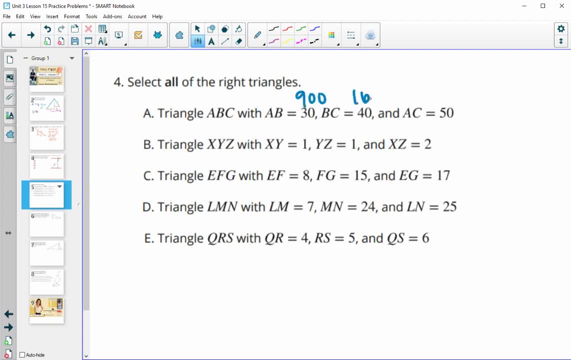 squared equals c squared. So we'll just square these all And then we'll compare. So the largest one has to be equal to the sum of the smaller ones, And that is true for this first one. 900 plus 1600 is 2500.. One squared is one. One squared is one. Two squared is four. One plus one does not. 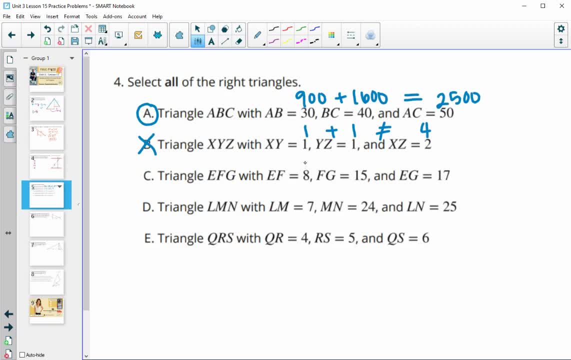 equal four. So this is not a right triangle. In c, 8 squared is 64.. 15 squared is 225.. 17 squared is 289.. 64.. Plus 225 does equal 289.. So this is a right triangle. 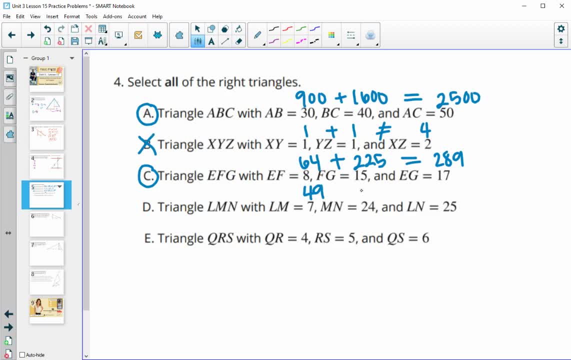 D, 7 squared is 49.. 24 squared is 576.. And 25 squared is 625.. 49 plus 576 does equal 625.. So this is a right triangle And the last one, 4 squared is 16.. 5 squared is 25.. 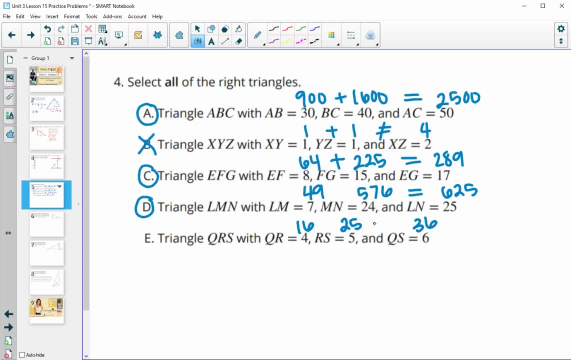 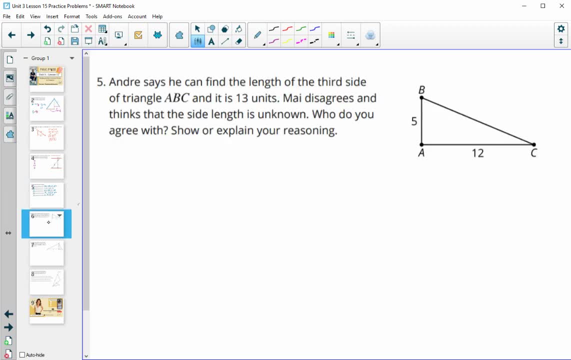 6 squared is 36.. 16 plus 25 does not equal 36.. So this one is not a right triangle. Number five: Andre says he can find the length of this third side, bc, And he believes it's 13. And Mai says that you can't find it, So she disagrees and thinks that. 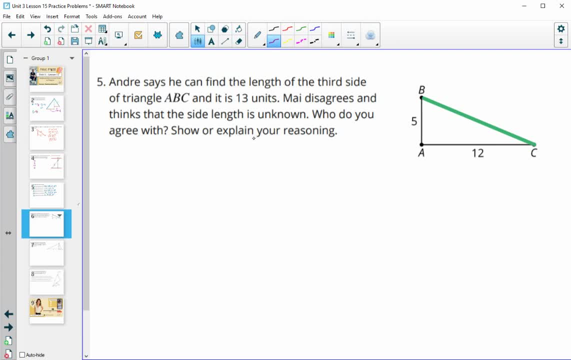 side length is unknown. Who do you agree with? Show or explain your reasoning. I agree with Mai, and that's because we don't know if this is a right angle. So, since we don't know if it's a right triangle, we can't use Pythagorean theorem, which is what Andre did. 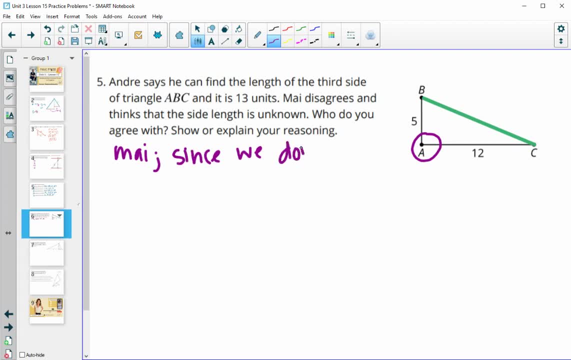 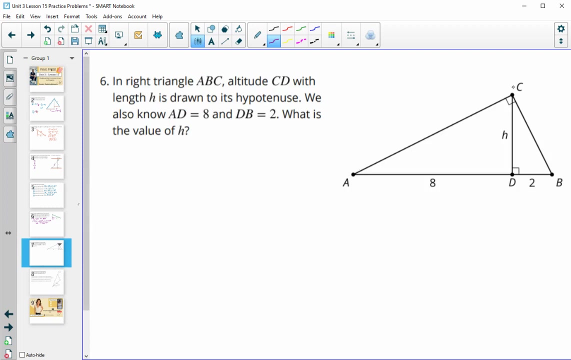 So since we don't know the measure of angle A, we can't use Pythagorean theorem Number six in right triangle ABC. so this large triangle here is a right triangle. CD is the altitude. We know that AD equals 8,, BD equals 10, so let's find the length of the altitude. 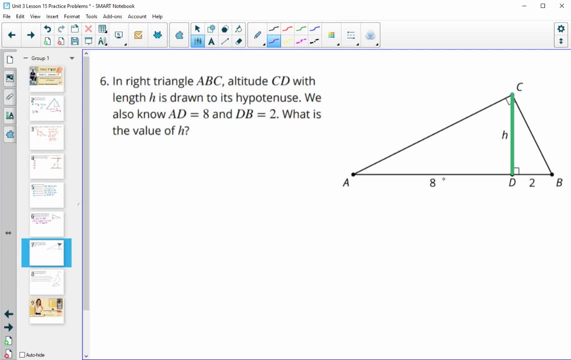 So we know that the altitude is proportional to these hypotenuse pieces. So we'll set up a proportion: 8 over the altitude, H equals H over the other hypotenuse piece, of B, And then we can cross, multiply, so we get 16 equals H times H, which is H squared. 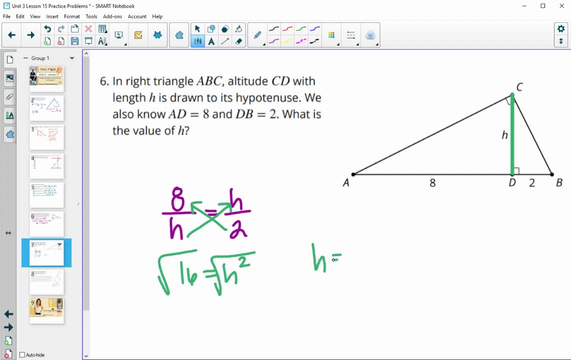 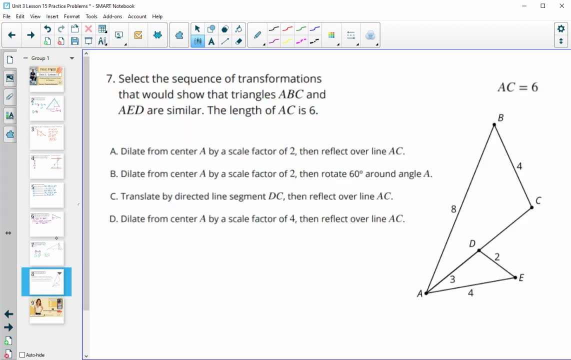 So then we can just square root both sides and we end up with H equals 4.. Number seven: select a sequence of transformations that would show that triangles ABC and AED are similar and the length of They're giving us the length of AC. 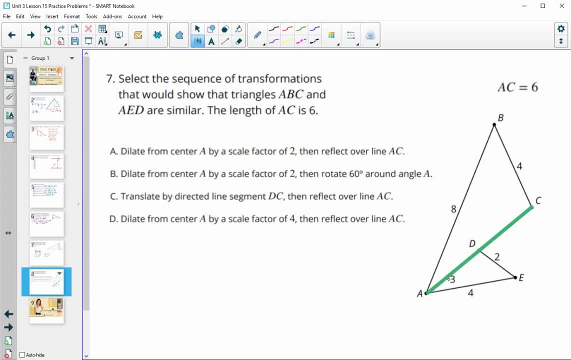 This segment here is 6.. So we see that this piece down here is already 3, so that means that this piece is also going to be 3.. Now I don't love the way that they wrote these, because they didn't tell us which figure we're dilating. 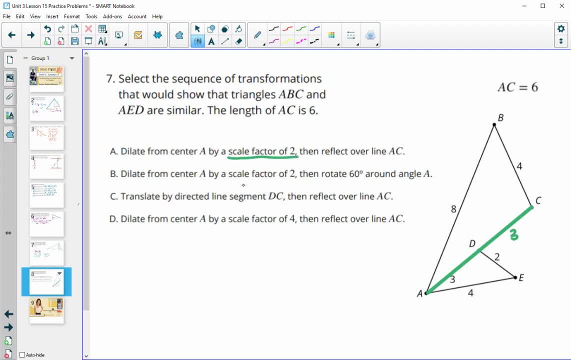 But since they say a larger scale factor or a scale factor larger than 1 in each of these, they are working with triangle ADE first. So they really should, In my opinion, say: dilate triangle AED by scale factor of 2..